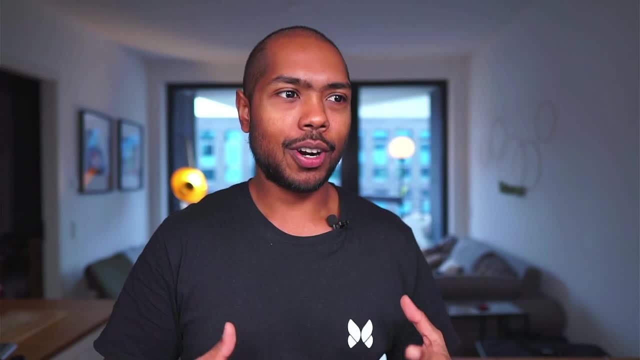 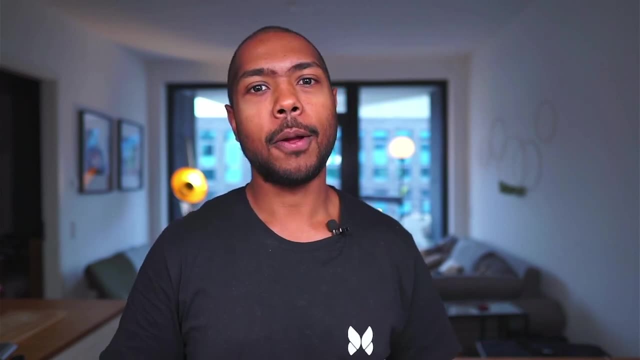 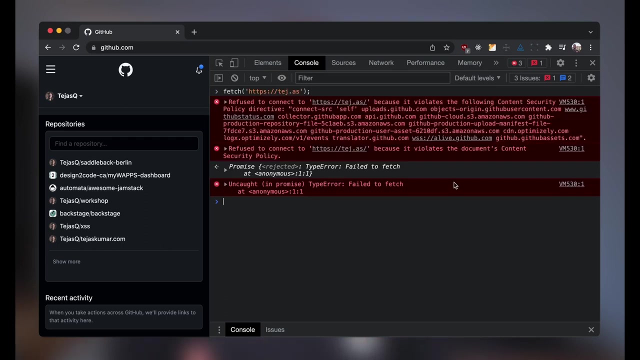 in a really granular way, describe what you allow, what content you allow and from where you allow it and how you allow it on your webpage. This prevents scripts from calling out to any other origin, Like this prevents somebody loading a script from like hackerscom on your website. 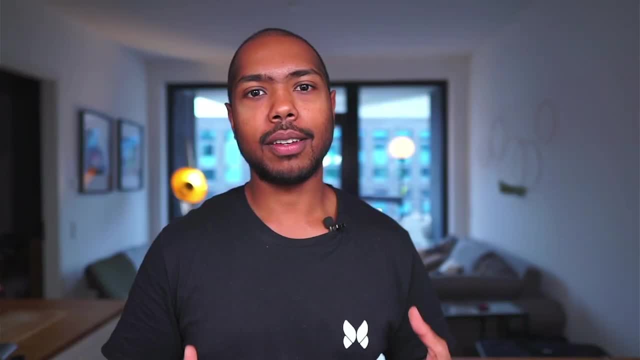 because your content security policy doesn't allow it. It's actually really great for fine grained control of what content your website is allowed to render or call. So it's a huge security benefit here. And so you might be thinking: great, that's fantastic, How do I use it? 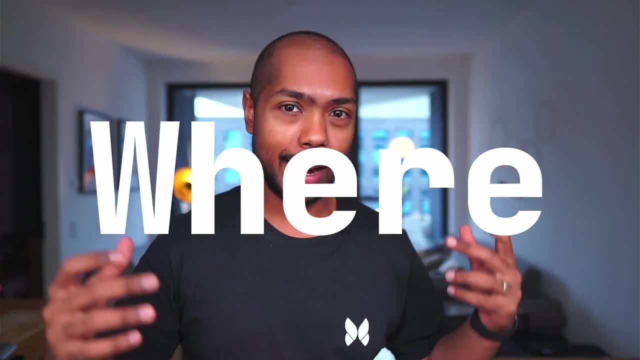 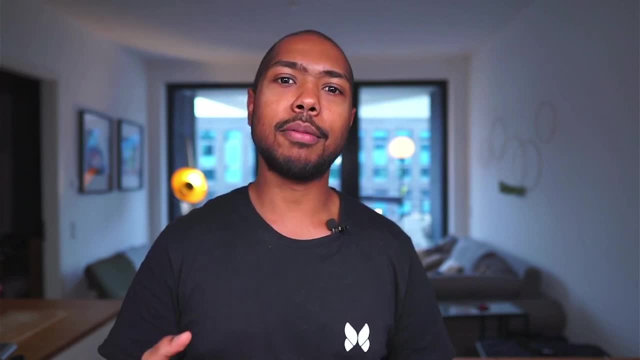 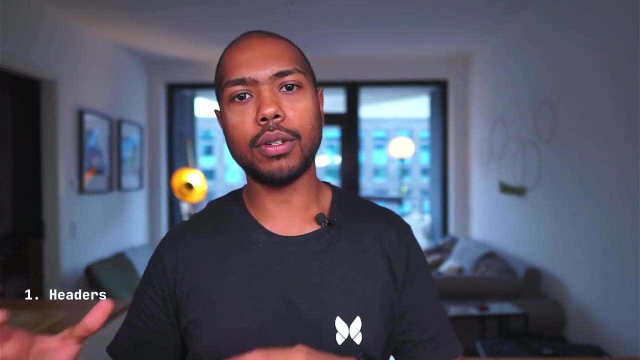 And before we talk about how, we need to talk about where I've seen content security policies being used, really in three different places And I'll list them in maybe descending order of frequency I've seen them used. The first is from a server, in headers. So when a server sends you a webpage, it includes with 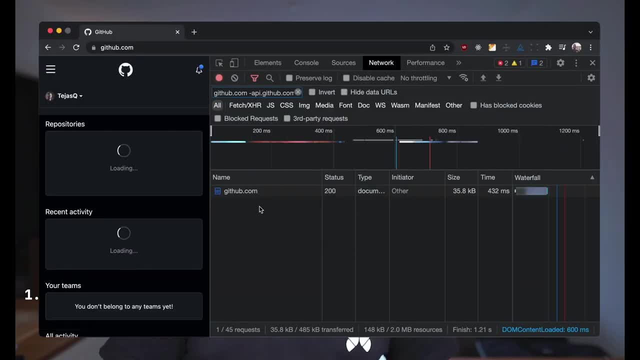 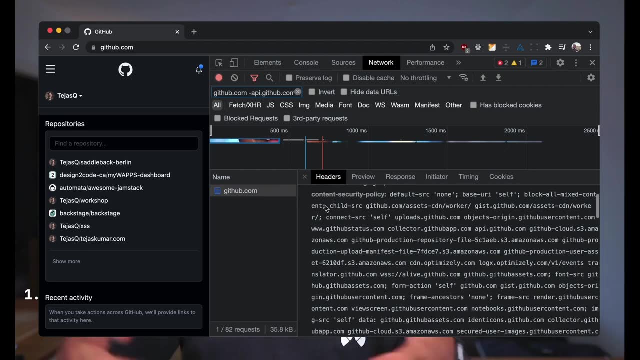 it headers, which is just a bunch of information about the server. For example, I'm sending you HTML page. by the way, I'm the server And this is my identity. by the way, I'm the server And this is my content security policy. So when a server sends you a webpage, it includes with it headers. 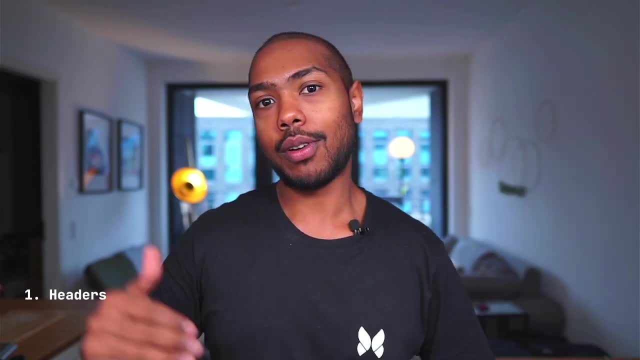 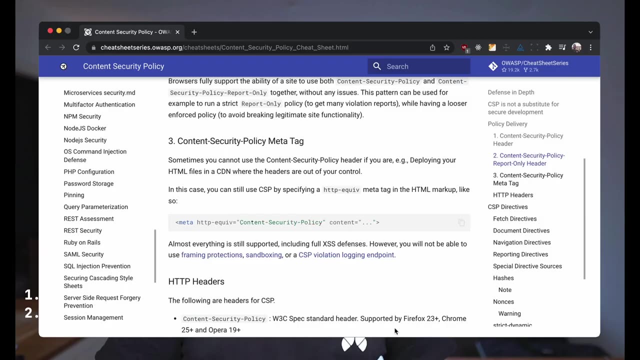 which is just a bunch of information about the server. So when a server sends you a webpage, I only allow scripts from this site, I only allow images from that side, and so on. So headers is one way. A second way is meta tags on the client side, But, as you can imagine, this has some limitations. 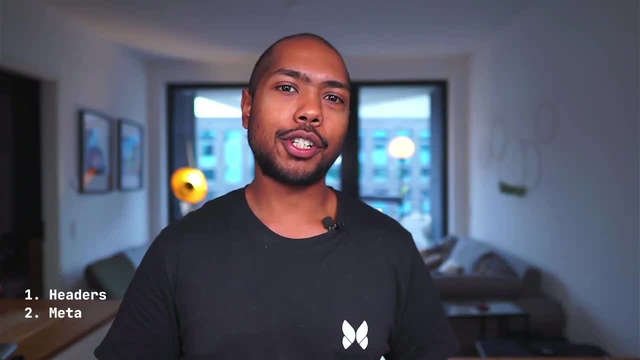 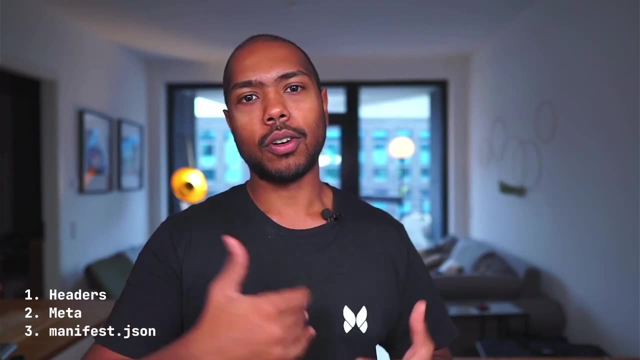 so not the best. And then the third way. I haven't really seen that much, but I think it's mostly to do with, like, Chrome extensions or something, And that is to include a manifestjson with your content security policy in there. I won't be covering that because it's not really common. 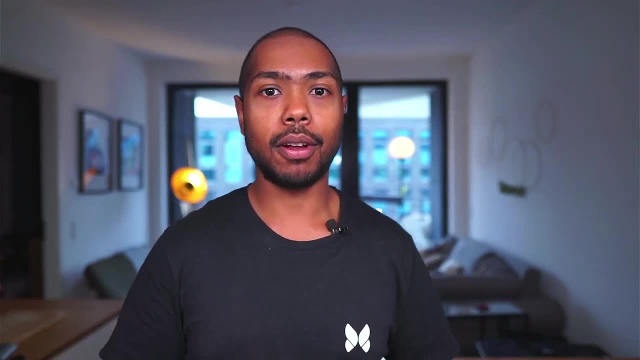 Now that we know where to put the content security policy, how do we do it? How should it look? Well, we've already agreed and decided to do it via server sent headers, So we have a header called content security policy. The value of this header is the. 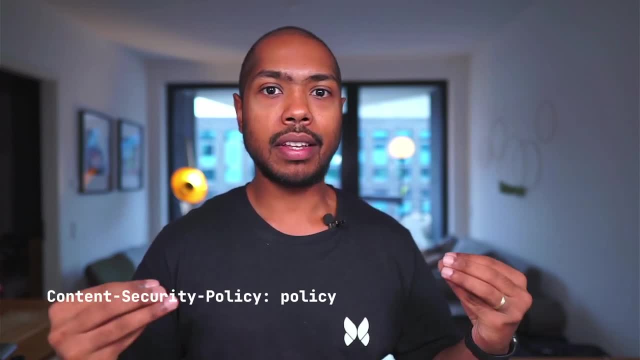 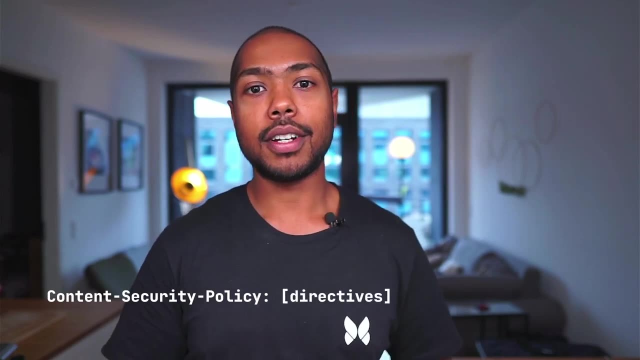 content security policy. It's how your website deals with contents from different sources. Content security policies are written using things called directives. There's many, many directives. We won't cover them in this video, but I'll add a link in the description. 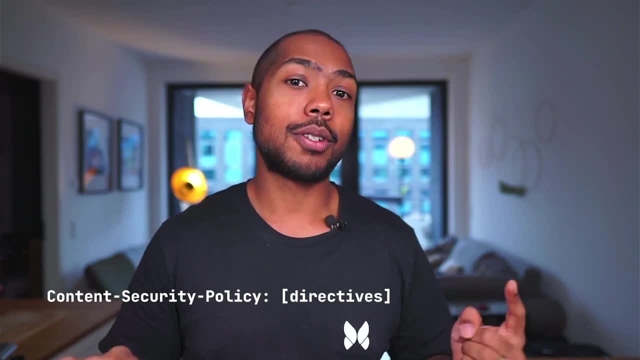 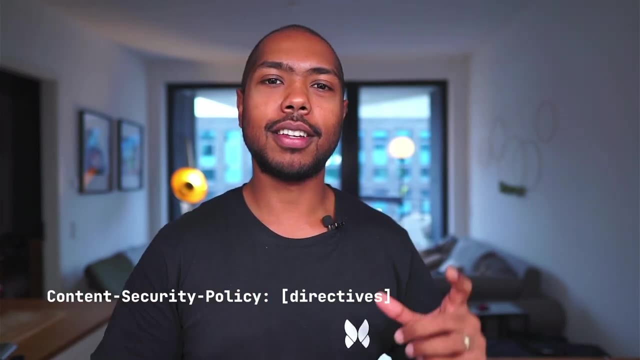 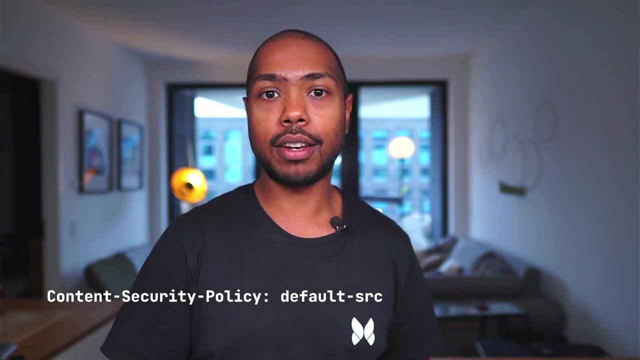 to maybe all the directives. We will talk about the most common directives And by far the default directive. the foundational directive, is called default source, default dash, SRC And this tells the page that is being rendered from your server sent content security policy. whatever happens, 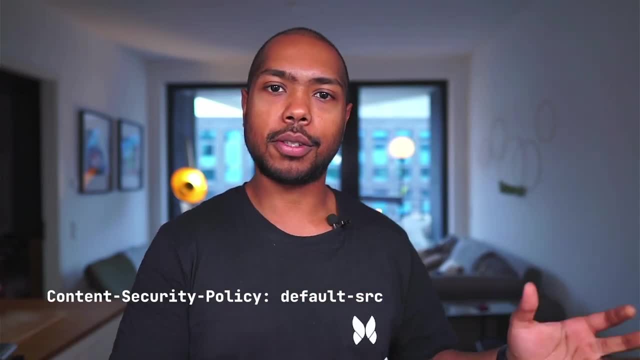 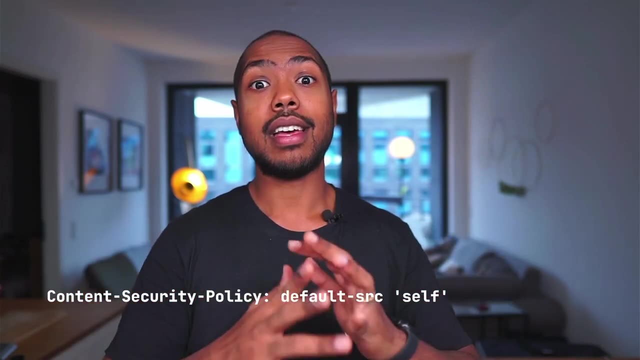 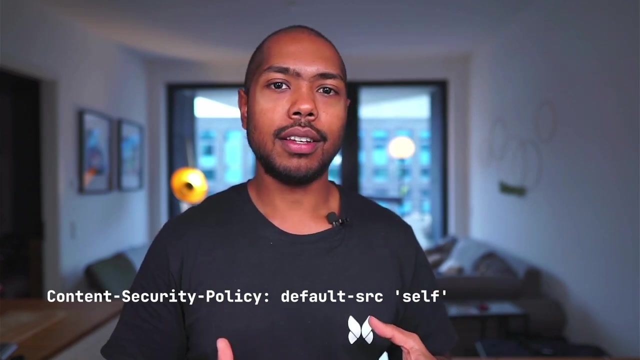 this is the policy for everything. So if you set default source to self in single quotes, that means I'm only going to load things from my own domain. Nothing cross domain is allowed on this page. It's already quite secure. You can then more granularly describe how you deal with scripts. 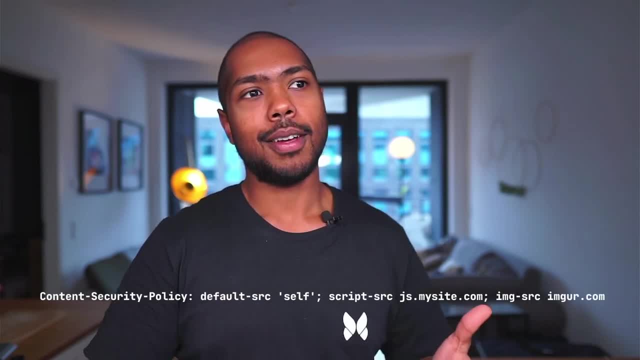 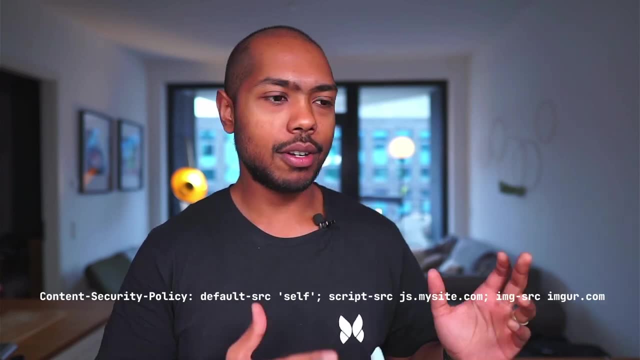 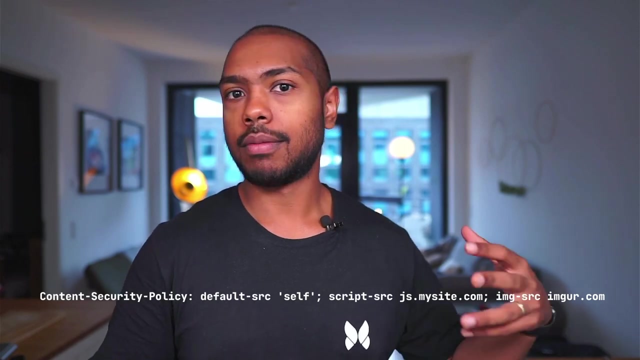 So that is JavaScript or images or media and so on and so forth, And you would delimit different directives in your content security policy using semi-colons. So you have a default source: self. semi-colon script source: scriptscom. semi-colon image source- imagercom. 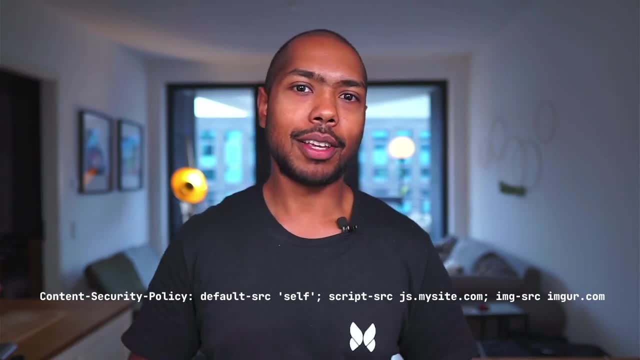 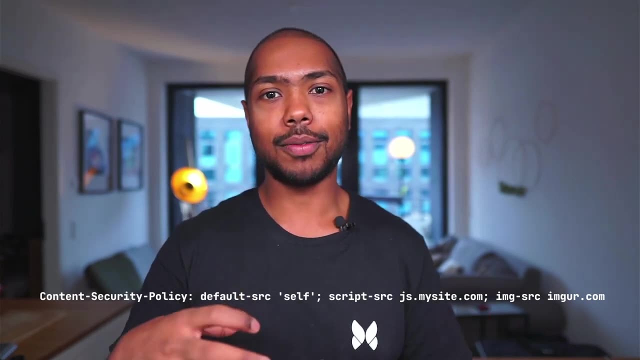 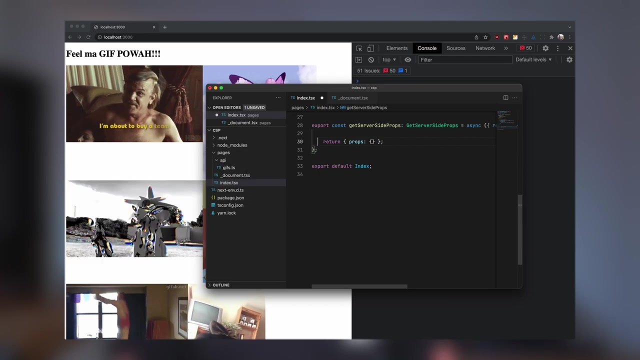 and semi-colon media source, whatever you like- youtubecom. I don't even know if you can do that, but that's generally the gist of it. So you have a default source and then you can change allowed sources per type of content, And that's how you do it. So these are the basics. Let's look at how. 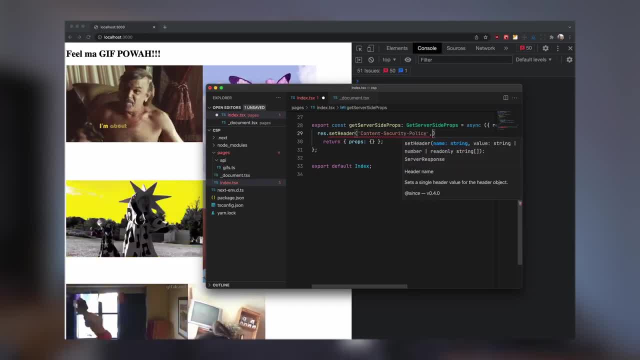 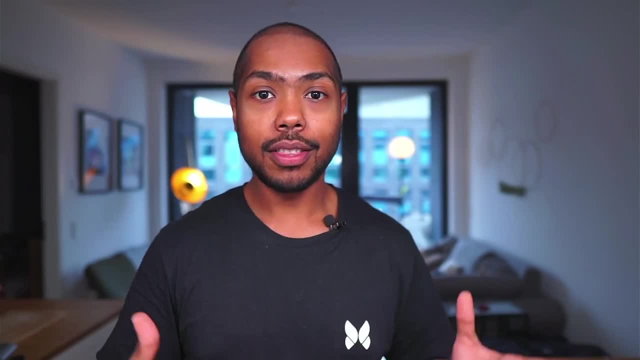 we actually implement one. So we'll add a header and we'll add some directives, But if we just send the content security policy like this, we might end up with a blank page, because there's a good chance that we have stuff loading in from a lot of other websites, especially images, as you can. 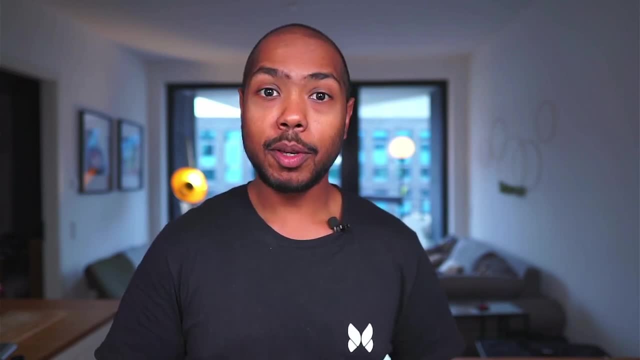 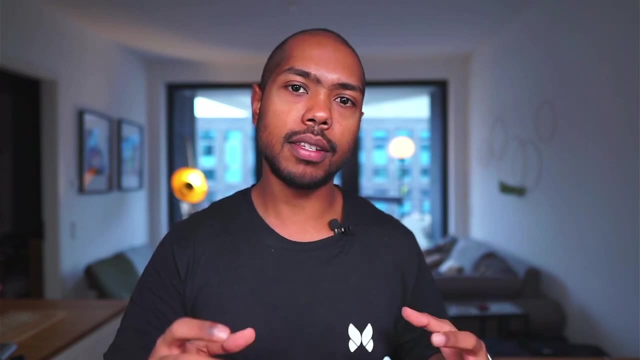 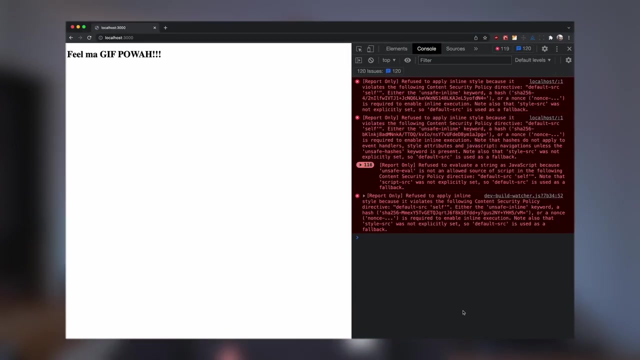 imagine. So maybe that's not ideal. Maybe we want to iteratively add this, And we can do that If we tweak our header just a little bit and instead of content security policy we change it to content security policy report. only then what's going to happen is the policy is still being sent. 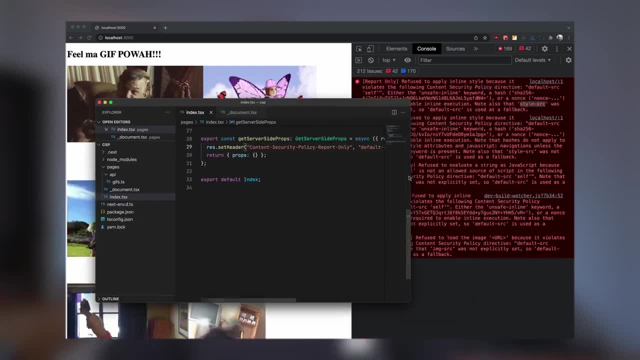 to the browser but is not being enforced. Instead, the browser just reports what violations happen. So then you can look from content made reports and then you'll be almost ready and able to wanna smell theueprint right away to understand what's going on in that argument. So you shouldn't have too 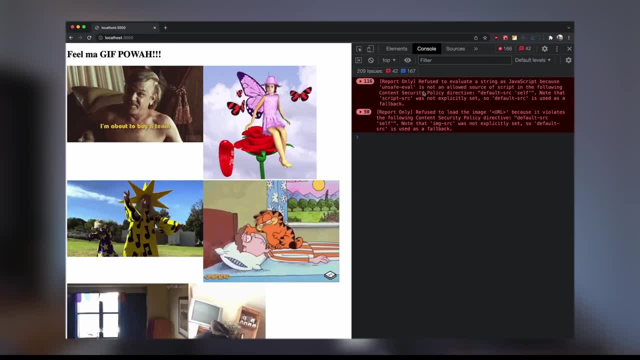 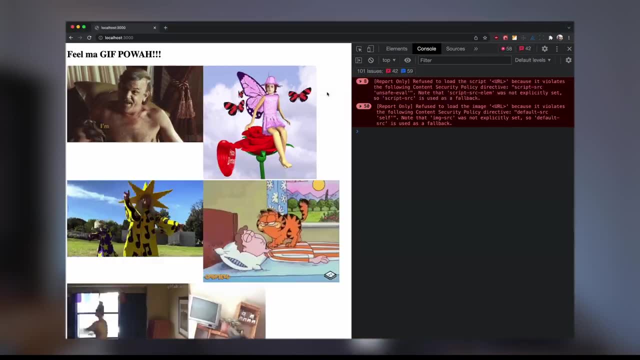 built in content security. So that's really해도 approaches. also, all these little things, we x them to a word within the code. then you can, at your console you can see what's not allowed and go tweak your content security policy as needed. and once there's no more warnings, once everything looks pretty good, you can remove the report. only.